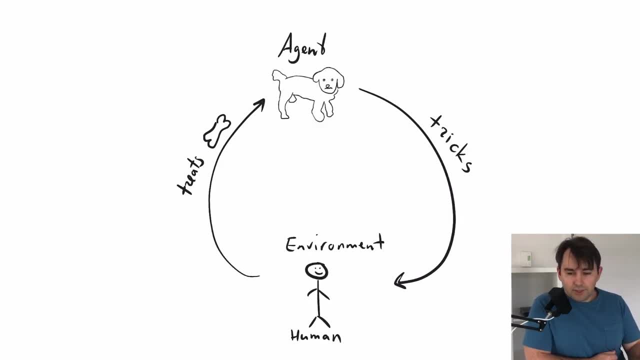 Imagine you have a dog that does something that the owner likes. Then the owner will give the dog a treat And the dog will tend to remember that this action leads to a treat and will do that action more often. Then the owner will give the dog a treat and the dog will tend to remember that this action leads to a treat and will do that action more often. 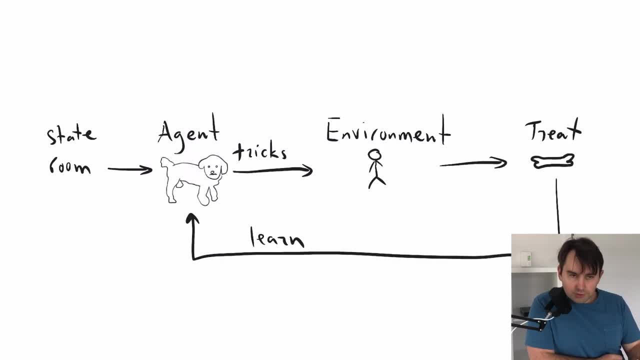 We can also draw this the same way we drew our environment before, to see how the learning happens here. And, as we can see, the dog uses the treat to reinforce those actions that the owner considers good. In other words, if the dog selects an action that results in good outcome, then it should. 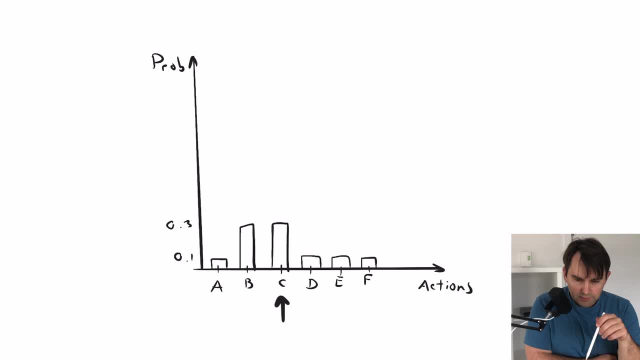 take that action more often in the future. For example, if the distribution of a possible action is as follows: and one of these actions turns out to lead to a good outcome, such that one of these actions, for example, returns large monetary reward of a thousand dollars, then we should kind of 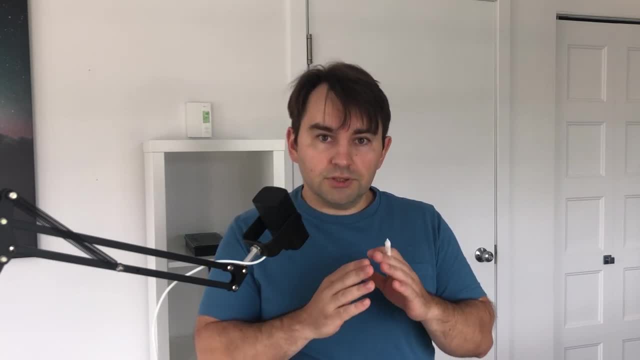 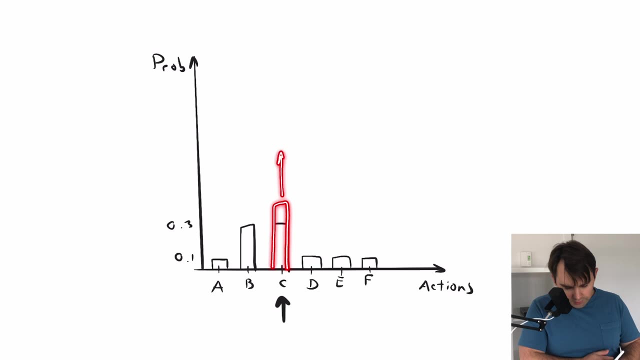 squish our distribution around that action such that that action happens more often. So we'll push this action up, we'll make this a bit higher, and we'll make this a bit lower, and we'll make all of these also a bit lower, lower as well, and this one as well. so we'll go and do it like this, and so the result is this. 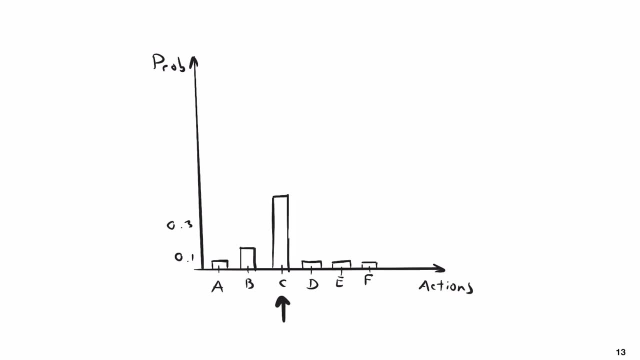 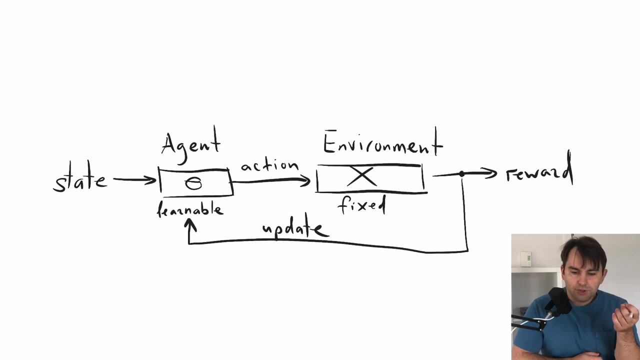 was our previous distribution and this is our new distribution. previous new. here you can see that this action c now has higher probability, so we pushed that up and brought all the other ones down. so more generally, we can use good or bad outcome as a signal for learning. this can be used anytime. 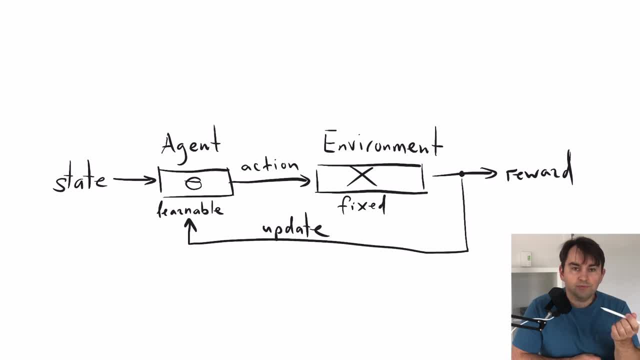 you have some goodness measure of your neural network output. so when you can't back, propagate or differentiate through the process that takes your output and hits it somewhere else, instead of using the gradient, as we normally do in supervised learning, we can just adjust our behavior in a direction. 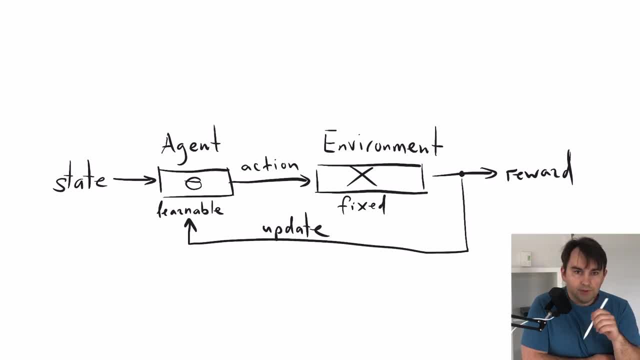 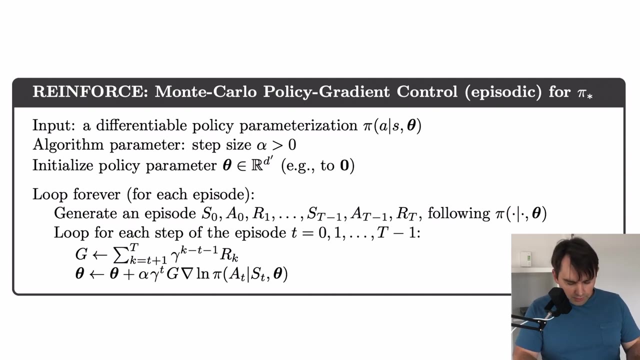 of the reward, and this is the key idea of the reinforce algorithm. it says that if we have something that we cannot differentiate, we use a reward as our signal to help us move the weights instead. so how does reinforce do that? let's take a look at the reinforce algorithm. the input to the 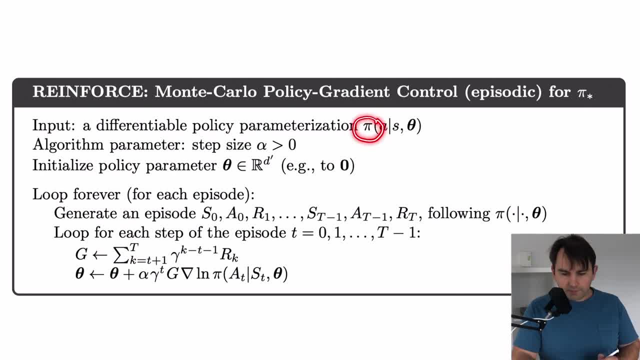 reinforce algorithm is some policy pi right here. so some policy that outputs an action given some state and it's parameterized by some parameterized data and it outputs some action, a. this could be our neural network. then we have a step size alpha, for example. this could be a step size for our adam optimizer. and this right here is just. 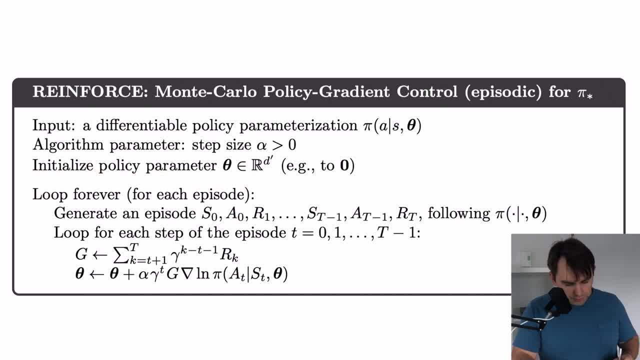 initializing our neural network weights. then we just loop over this part forever, right here. so inside our loop we have our policy to generate the full episode. so from state zero we use our policy to produce action. a zero the environment takes our action and outputs the next state. 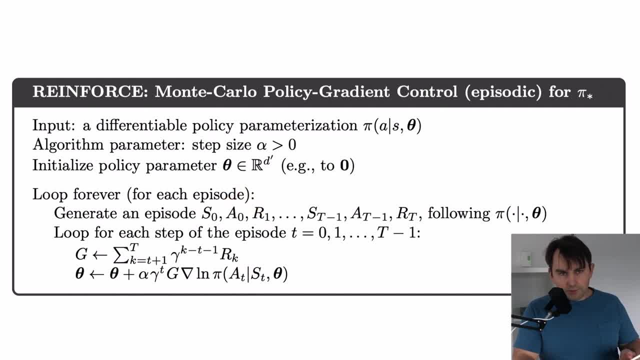 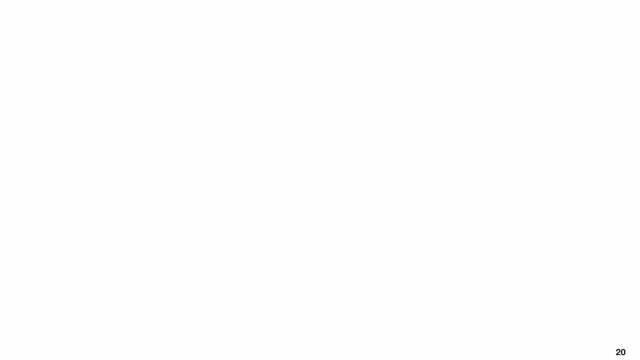 s1 and the next reward r1. we continue this over and over until we get to the terminal state and terminal reward. so notice that so far we haven't done any learning. we just used our policy to generate a trajectory, starting at some state at zero, going to some state. 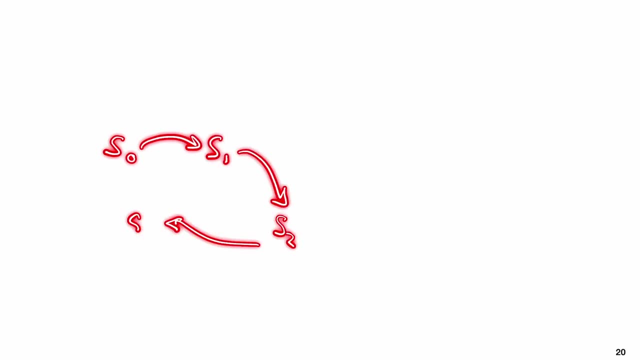 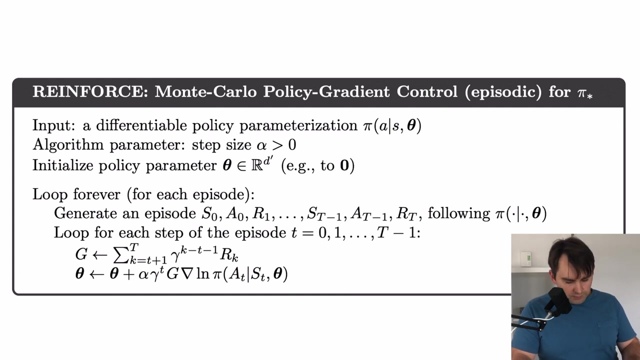 state S1,, S2,, S3, perhaps over here to S4, until we arrive at some terminal state. And all of this is done using our policy Pi. So once we have this full episode of experience, we can loop over each time step of the episode right here and we compute our discounted return. Discounted return is just. 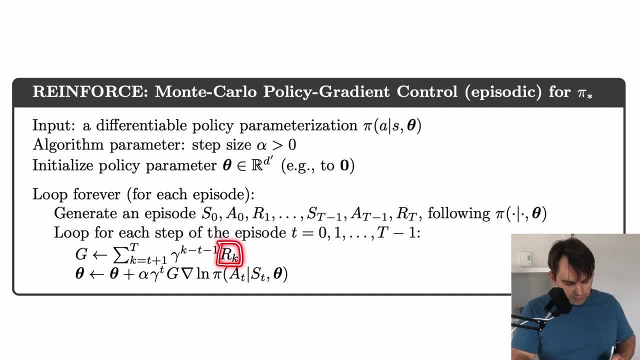 sum of all the rewards, starting from this Step K up to the final time step, multiplied by this discount factor gamma. and this discount factor just takes higher and higher powers as we progress into the future Once we compute our discounted return here, for every time step we multiply. 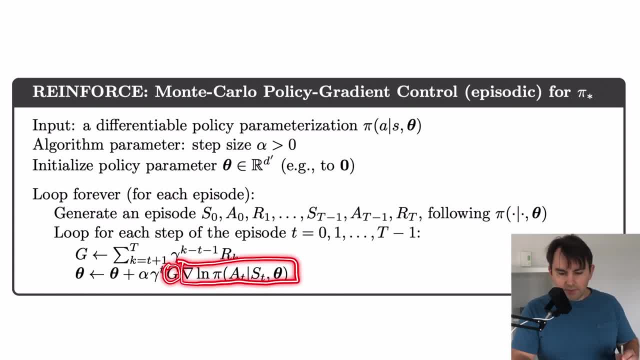 it right here by this other quantity right there, And this other thing is the gradient of the log of the Pi. This is the gradient of the log of Pi, And the gradient of the log of the Pi will be I policy. In other words, we take the output of our policy right here, compute the log. 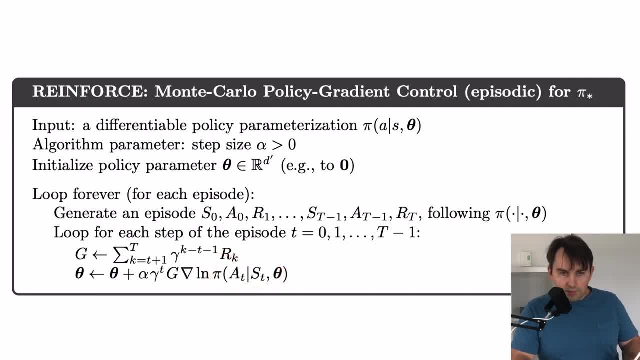 of it and then compute the gradient. This is what we multiply our G term by. But looking at this and trying to figure out what happens is kind of tricky. so I'd like to get you to focus on two things. First is how to sample an action and the 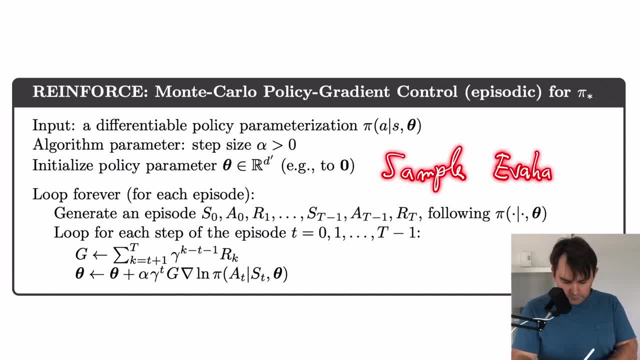 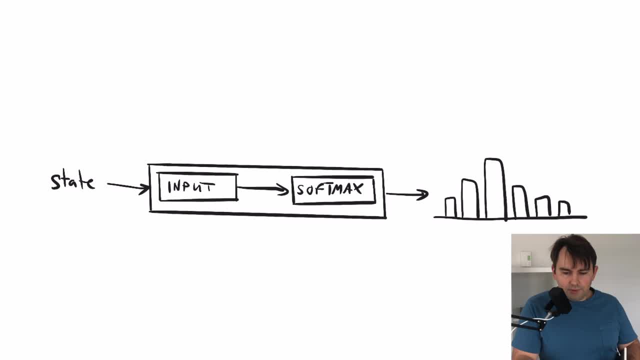 second is how to evaluate an action. So to get the action, we sample it, meaning we take our state, feed it into our policy and we get the softmax over possible actions. This forms a probability distribution right here. Then we sample an action from this distribution and, as you can see, some. 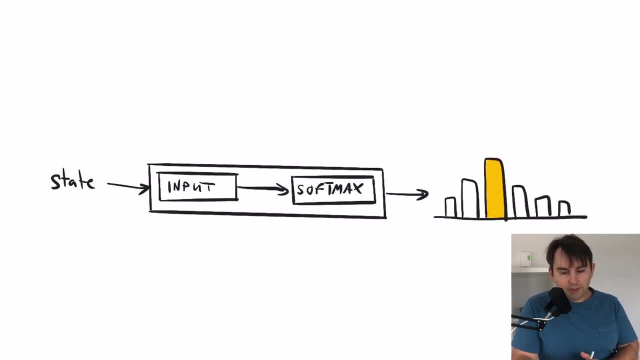 actions are more likely to be picked, while others are more likely to be picked. So we sample an action from this distribution and, as you can see, some actions are more likely to be picked, while others are less likely to be picked. Regardless, once we sample our action, we have a 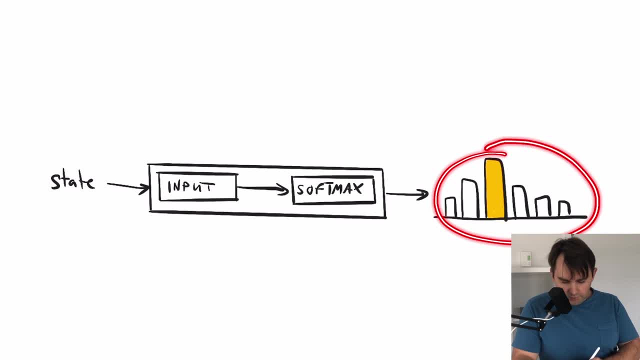 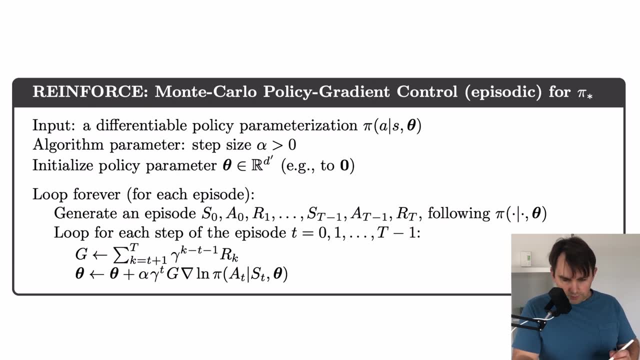 concrete action. So in this case, perhaps we sampled the yellow action because it was more likely. So in our algorithm this is done right here. We're constantly sampling an action from this policy, and the action we sample produces a concrete action right here, A, which we can then give to our environment. Next the other. 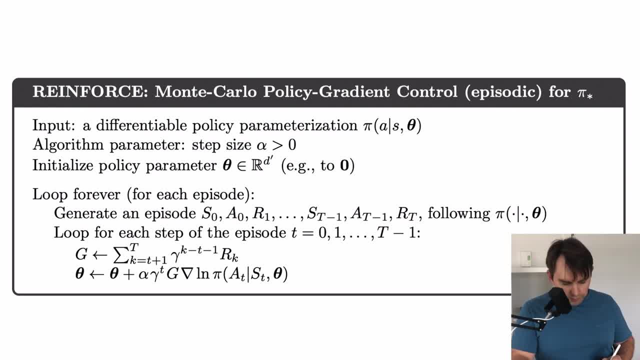 thing I wanted to note is that we're going to be sampling an action from this distribution because it's in the correct order right here. Next, the other thing I' d like to notice is how we use this action. Yes, one way we use this, it's. 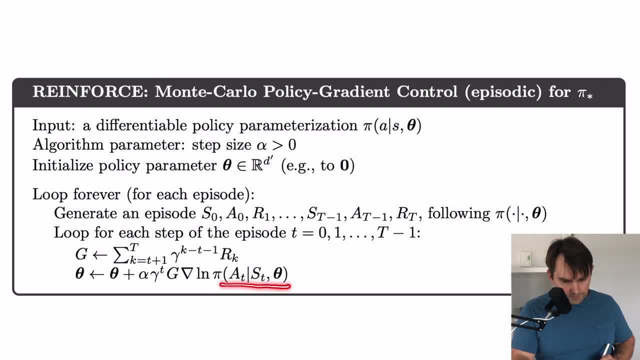 right here when we give it to our environment. but this is not what I'm talking about here. What we're interested in is when we use our action right here. But our policy outputs an action, and here it seems to actually take an action as an input. So 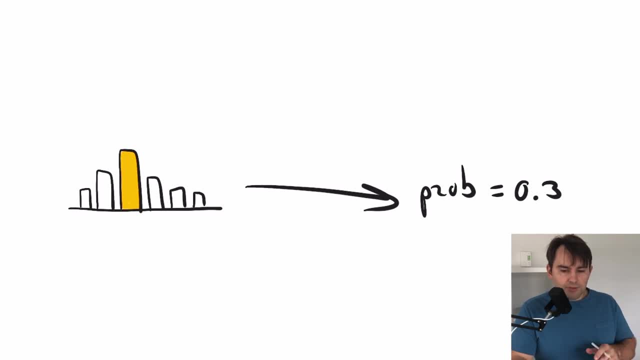 the first time you look at this, you're confused. Actually, what we're doing here and finding the probability of that action in our distribution. So this is our concrete action: we selected and the probability of selecting it is 0.3,, for example, 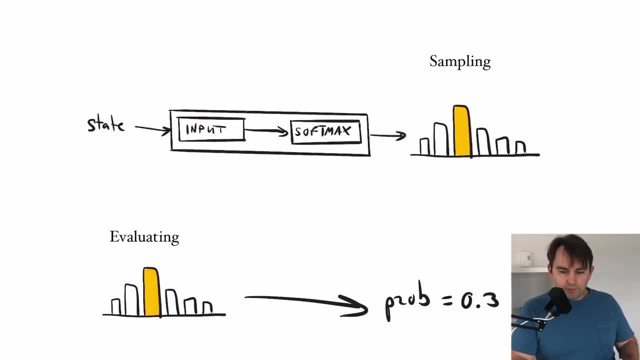 This is called evaluating, Unlike the previous thing we did, which was called sampling, this is called evaluating. But how do we do this in code? This is just showing it in theory. Well, we can use PyTorch to help us sample and evaluate these things. 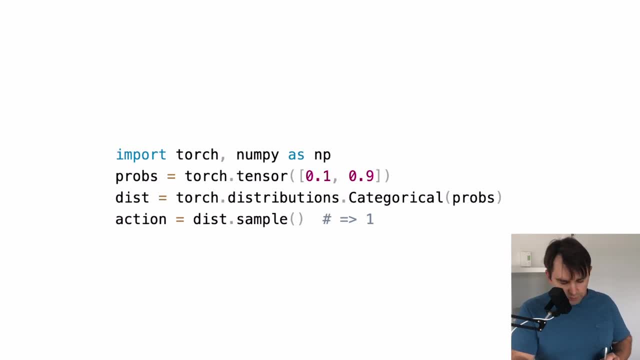 For example, we can use the categorical class from Torch distributions, which takes a list of probabilities and builds a distribution for us. We can then sample this distribution to get our action. Don't forget, this is zero-based indexing, so number 1 here. 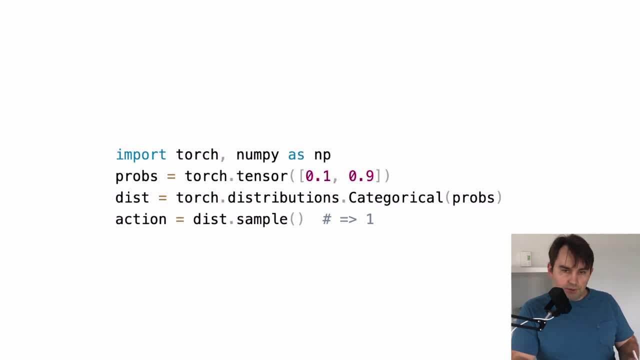 It means the second element was chosen because it had the high probability. After we sample from our distribution, we can evaluate a given action using this log prob function. For example, in our case we sampled action 1. So the probability of that action is 0.9.. 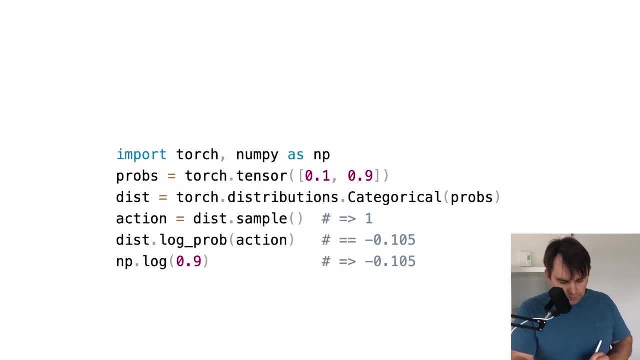 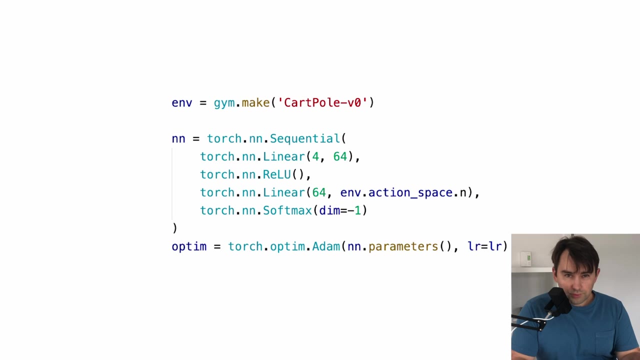 After we take the log, we get negative 0.105.. And we can verify that this is the case by taking the log of 0.9.. Let's now go through the implementation of Reinforce step by step. First, we declare our environment. 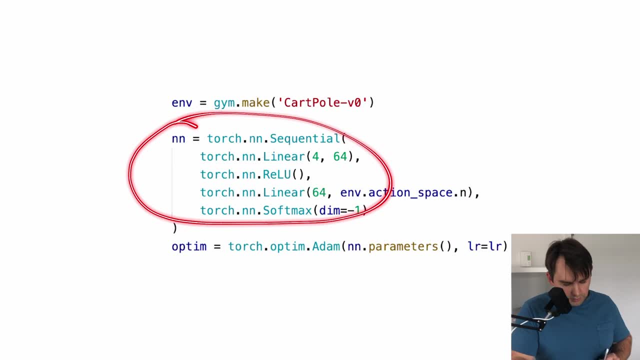 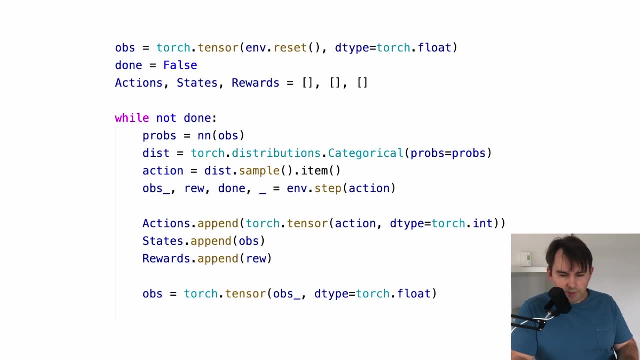 then our neural network and then our optimizer. Next, we gather one episode of experience. As you can see, what we're doing here is simply passing our observation to a neural network right here, Gating our probability distribution right here. 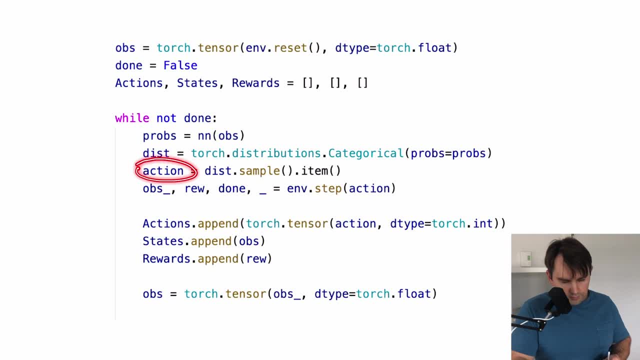 And sampling from it to get our action right here. After that, we use our action to take a step in the environment. As all of this is happening, we store all of the action, states and rewards in these arrays, So we're storing the history of things happening. 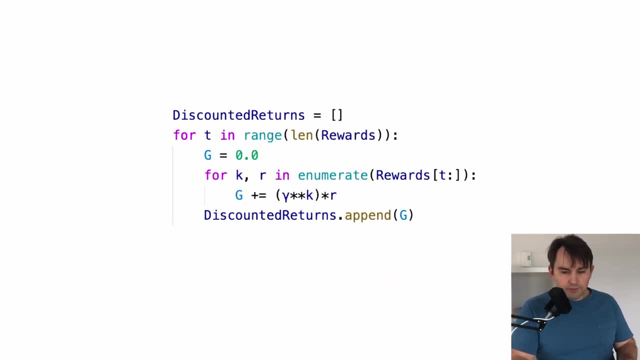 We will need them later. Next, after we collected our one episode of experience, we loop over the rewards in that episode and compute the returns for each time step. So, as you can see here, t represents 1.9.. t represents a time step at which we want to compute our discounted return. 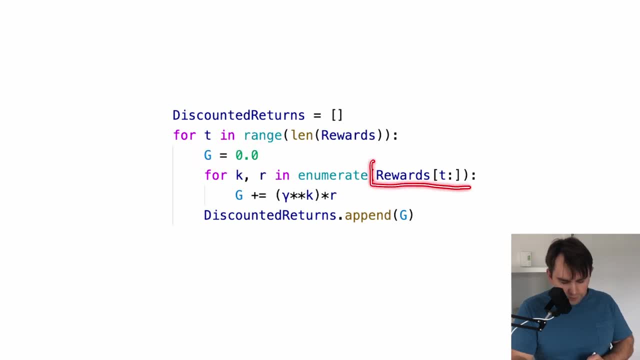 This is the discounted return for time step t. We just take rewards starting at that index and then iterate over them and multiply rewards by discount factor gamma to the power of k And you can see that this k always starts at zero for every time step. 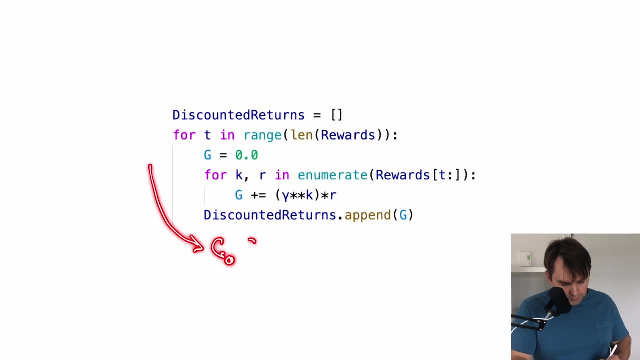 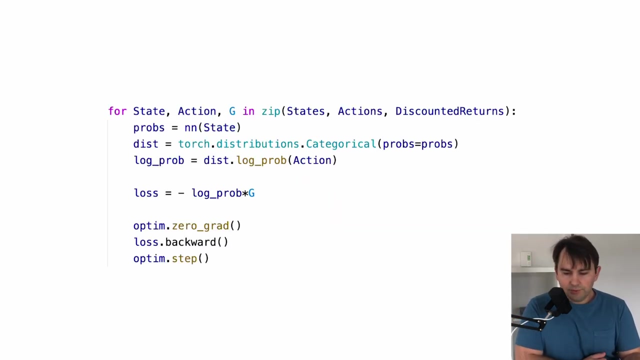 And so at the end of this we have a bunch of g's. We have g, g1, g2, g3, etc. And so we have our array of discounted returns. After we computed our discounted returns, we iterate over our episode again and update our policy at every step.